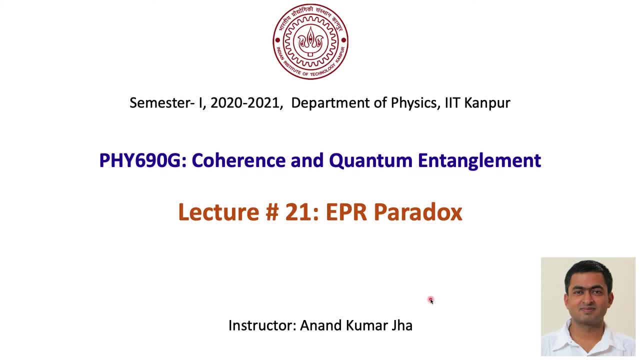 Welcome to lecture number 21.. So in this lecture we are going to study EPR paradox. EPR stands for Einstein, Podolsky, Rosen. There is actually no paradox here as such. It was just that in 1935, after quantum mechanics was kind of proposed as a theory, Einstein, Podolsky and Rosen- they 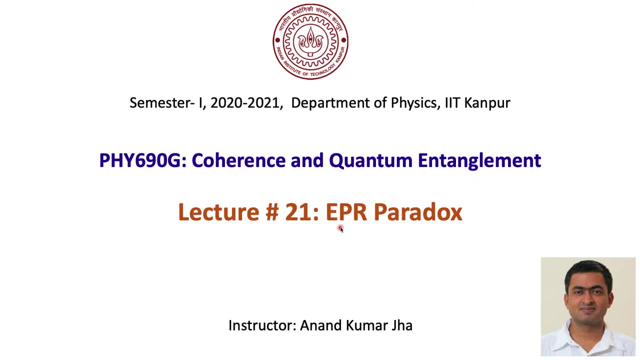 pointed out certain features of quantum mechanics that were kind of mutually contradicting each other, and that's why this came to. this is also referred to as EPR paradox, But essentially in this Einstein, Podolsky and Rosen were just questioning the quantum theory as a complete. 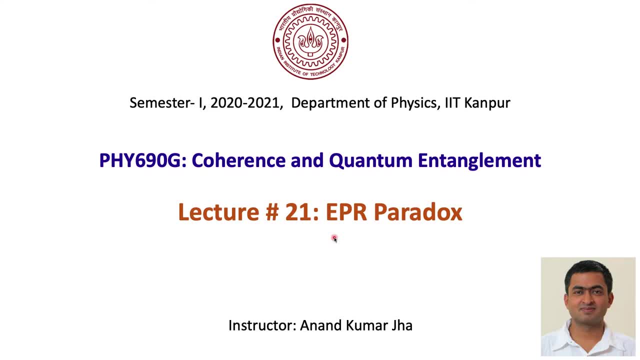 theory, or whether quantum mechanics is indeed a complete theory or not. So that's what we are going to study in this lecture. So that's what we are going to study in this lecture. So that's what we are going to study in this lecture. 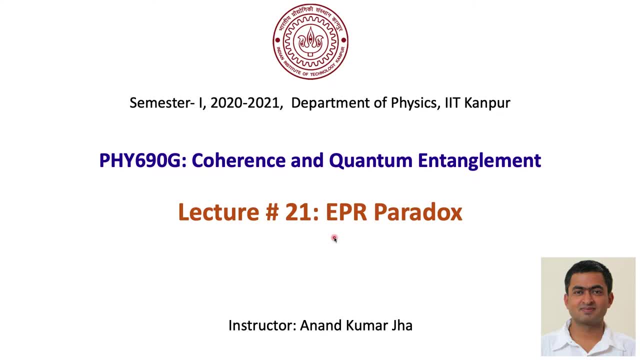 EPR. we are questioning, through few arguments that they pointed out and that basically sometimes is referred to as EPR paradox. So that's what, and this will be the starting point of defining entanglement in various degrees of freedom. So let's first look at what we did. 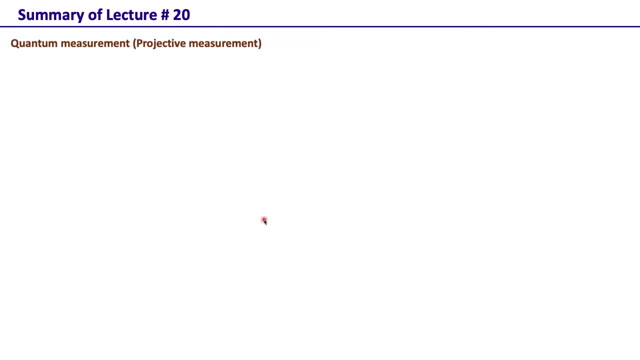 in lecture number 20.. So in lecture number 20 we did quantum measurements and specifically the projective measurements. There are two other kinds of measurements but we mostly looked at projective measurements. So for a given operator A, an operator, measurement operator always corresponds to some dynamical variable. So for that operator A, if it acts on a state, then the 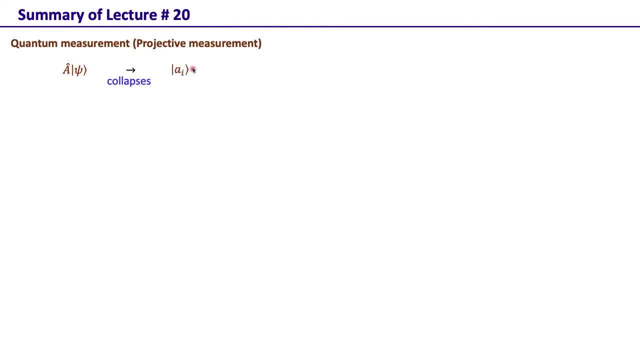 system in that state collapses into one of the eigen state of the system in the basis of the measurement operation. So for that operator, if it acts on a on on a state, then the, then the system in that state operator and one obtains the eigenvalue a and the probability of this collapse is given by 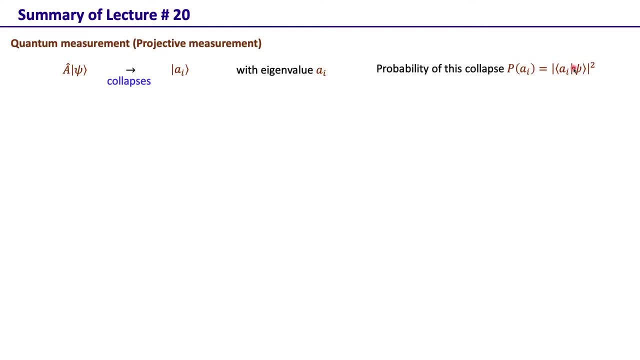 the mod square of the projection of the state on the i, the basis vector, or the eigen k, the, the probability, p, a, i, that is, of the collapse. that measurement of the observable yields the result a, i, this, this. then we saw that it can be written as this psi and this pi i operator. 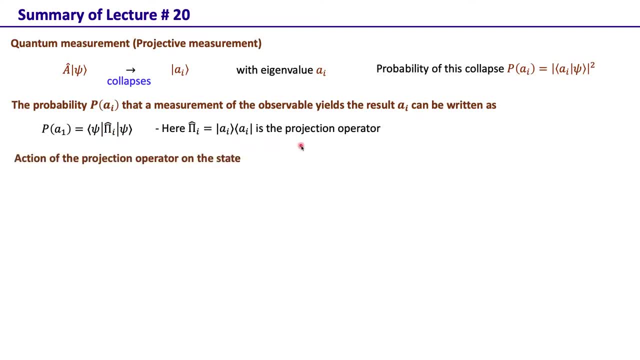 psi, and this pi i is the what's called the projection operator. we also saw the that. specifically, we saw that if we using this projection operator, if we act this on the state, then of course it yields the particular eigen ket. so this, this pi that there can be n such 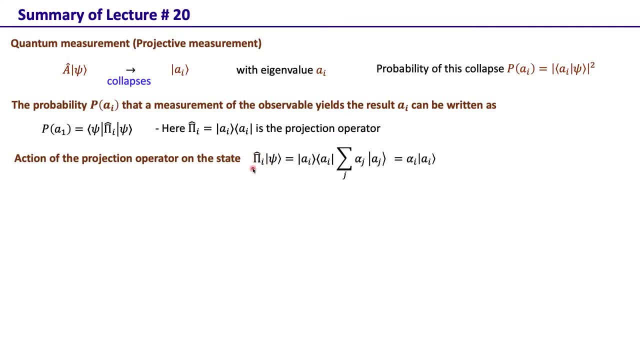 projection operator for an n dimension, n dimensional system, and and a pi i projector basically yields the eigen ket a, i and, of course, sum of all these projection operators is equal to one and and if it's a if, if this is for the discrete system, discrete basis, but if it's a continuous variable operator. 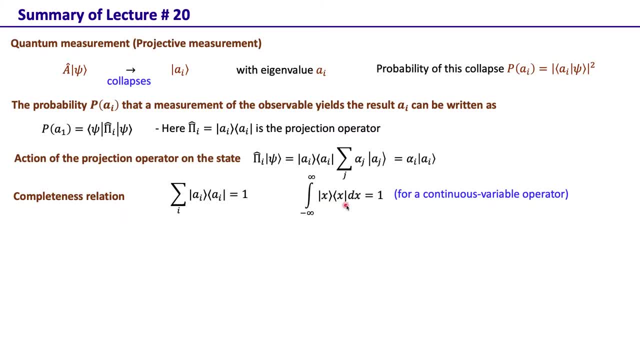 then this completeness relation reads as: x: x. this is for the position basis, so that's just an integral here. so the, the operator itself, can be represented in terms of these projectors in this manner. so a is a, i, that's the eigenvalue, and the projectors, and this is sum over these from. 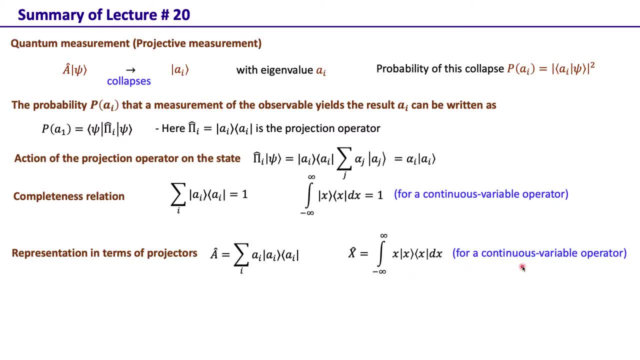 i equal to one to n, if it's an n dimension basis and for a continuous variable operator, then it's just an integral in this manner. so a measure when, whenever we talk about measurement, then we also looked at: whenever we talk about measurement, we- this is always a particular 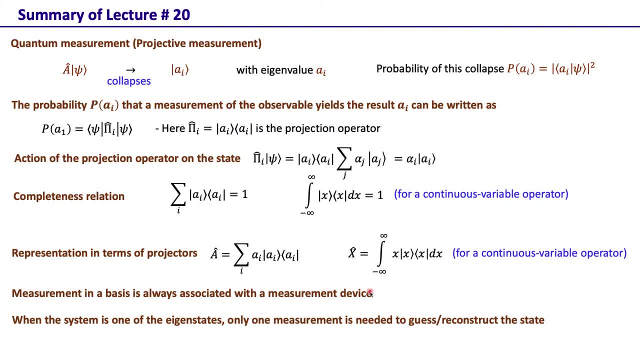 associated with the measurement device. for example, we saw that polarization is associated with polarization in horizontal vertical basis, is associated with the polarizing beam splitter in the horizontal vertical basis that splits a light field based on its polarization in the horizontal and vertical directions and similarly, like a lens, is a measurement device. lens, along with the 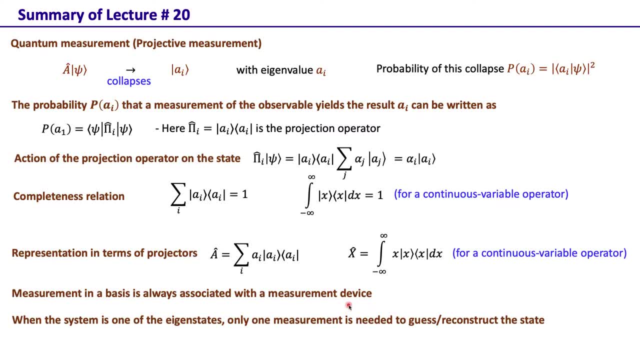 CCD camera can be measurement device for a momentum, a CCD camera itself can be measurement device for position, and so on. so now the aim of quantum. one of the aims of quantum measurement is to be able to find or predict or reconstruct the, the quantum state. unknown quantum state, and but if one knows that the 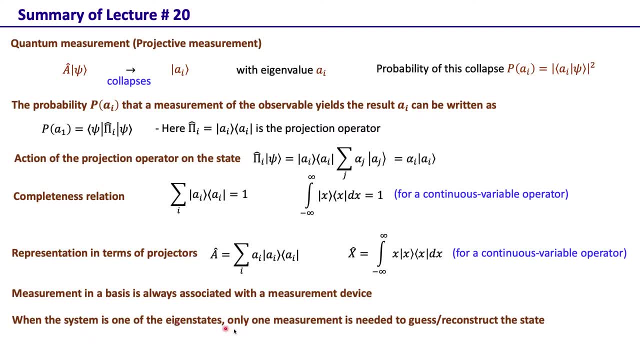 incoming quantum state is in one of the eigen states, then only one measurement is needed to guess or reconstruct the state in any basis. so we actually saw this explicitly for the polarization basis, but this is true in general that if the system is known to be in one of the 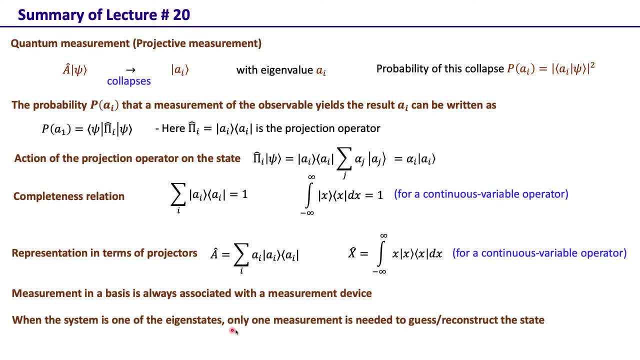 eigen state of the measurement operator, then only one measurement is required to reconstruct the state. but of course, if the system is in a superposition state, then one requires an infinite number of measurements to actually reconstruct the whole state. okay, so this was quantum measurement. now let's get to. 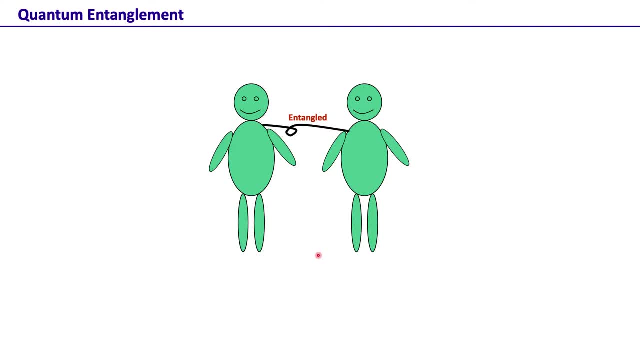 quantum measurement- EPR paradox. so let's get started with quantum entanglement. I have shown this slide earlier as well, so this is- this is a popular interpretation of quantum entanglement: that if two, if there are two entangled particles and if we disturb one, both of them actually get disturbed. this is actually not. 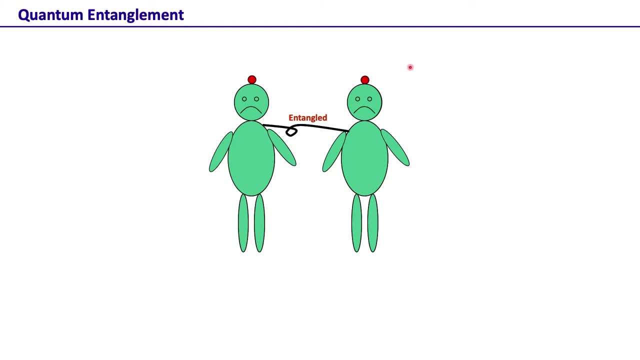 absolutely correct. but I like to show this because this kind of conveys the idea in a much simpler manner. but we will see. we will see in this the concept of entanglement in in a much more mathematically rigorous way, but this, this very idea of entanglement, this was. 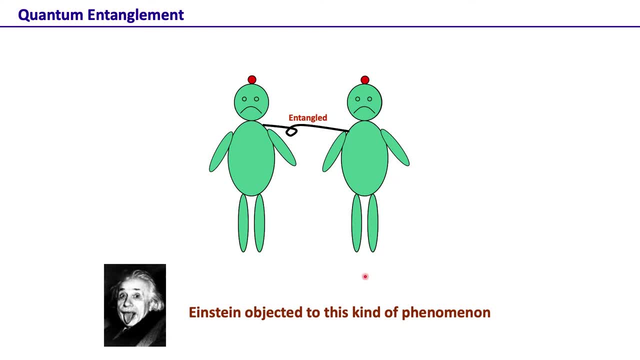 not really liked by Einstein- Einstein, podolsky-rosen to be specific- and- and they basically objected to this kind of phenomenon, and in this lecture we will actually look at and go through the exact arguments that they provided in order to kind of argue as to what was wrong with this very concept of. 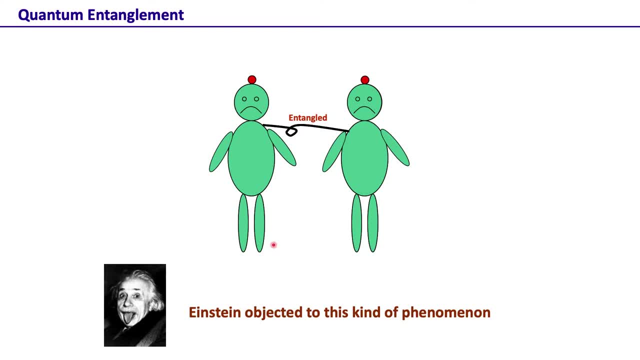 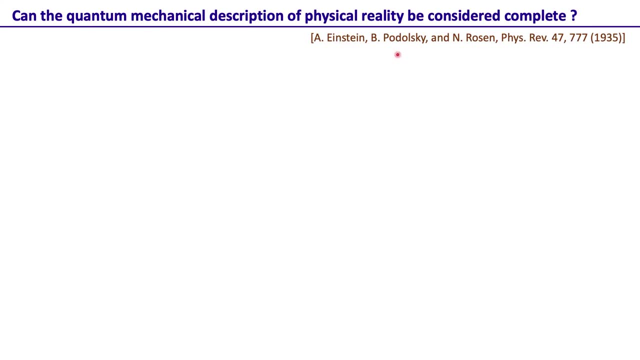 entanglement, in fact, what was wrong with the very quantum theory itself? so this was the paper that Einstein, Podolsky and Rosen- they published in 1935. this is a very famous paper and basically, in this lecture I am going to follow the exact formalism of this paper and this paper, in fact, this is: 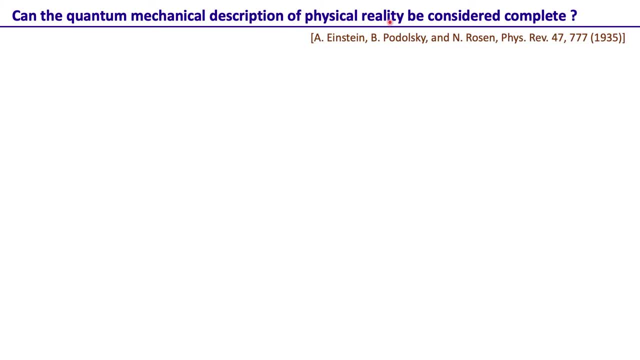 the title of the paper, that can the quantum mechanical description of physical reality be considered complete? so here they are basically questioning the completeness of quantum theory and of course, as I pointed out, this is also kind of referred to as EPR paradox. but essentially in this work they question the very completeness of quantum theory. so we will go through the 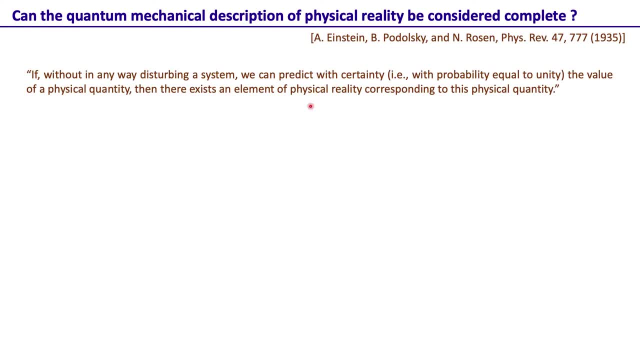 exact arguments, but here are the few statements taken directly from this paper that gives a a kind of overall view of what they were thinking of quantum mechanics at the time. so they say that, if without in this is just quoting EPR from this paper, if without in any way disturbing. 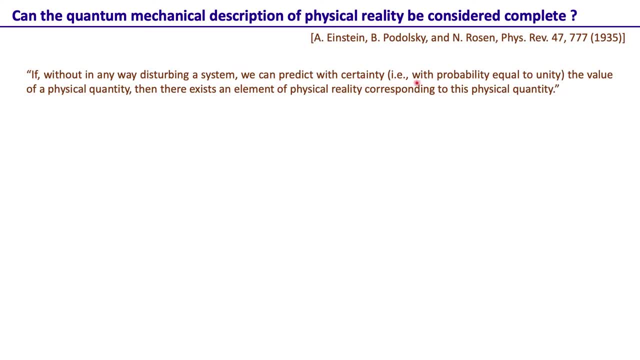 a system we can predict with certainty, that is, with probability equal to unity, the value of a physical quantity, then there exists an element of physical reality corresponding to this physical quantity. so here they are basically referring to the fact that the fact that the measurement should be certain, that one should be able to predict something with 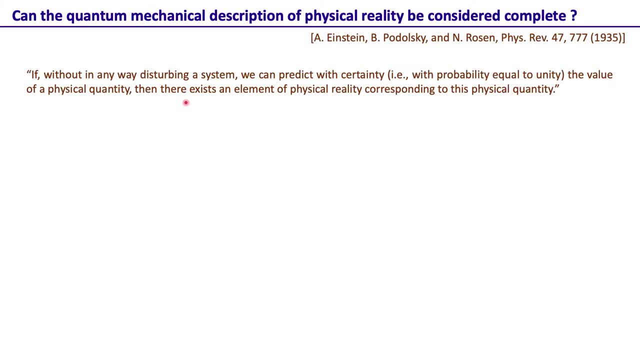 equal probability. and if that is the case, then only we can say that there exists an element of physical reality. essentially, here they are questioning and here they are defining what should be the idea of physical reality, what should be the requirement for something to be physically real. then they say that in a complete theory there is an element corresponding. 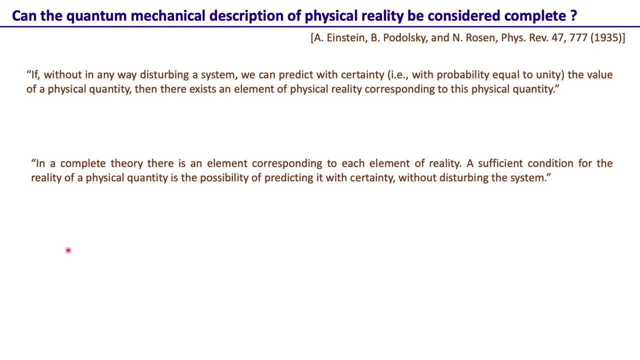 to each element of reality. a sufficient condition for the reality of a physical quantity is a possibility of predicting it with certainty without disturbing the system. so here they are defining what should be the element of reality, and for that their main argument is that for reality, one has to be able to predict it with certainty without disturbing the system. 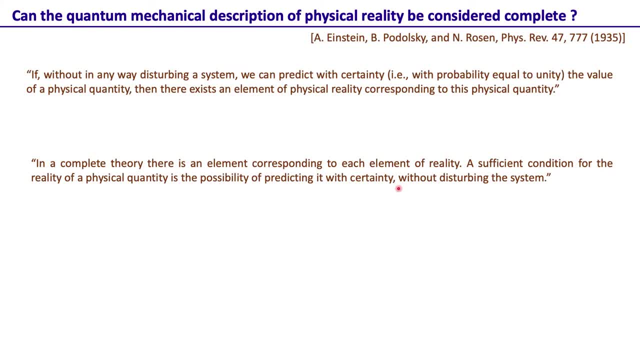 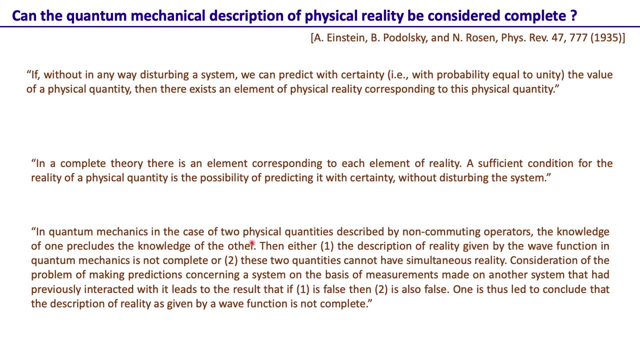 and disturbing the system. So which one is the solution for this? Well, it might be that the system should not be a kind of a part of that definition. then, finally, they argue that in quantum mechanics, in the case of two physical quantities described by non-committing operators, the knowledge of one precludes the knowledge of the other. 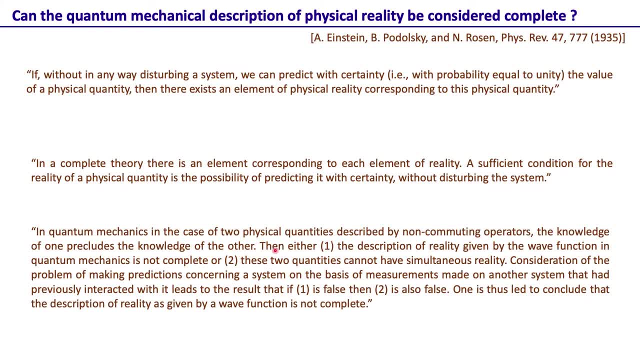 here they refer to the fact that we have a for non-committing operators. we have uncertain relation in the sense that if we know one very precisely, the other one cannot be known with arbitrary accuracy. So then they say: Either one. the description of reality given by the wave function in quantum mechanics. 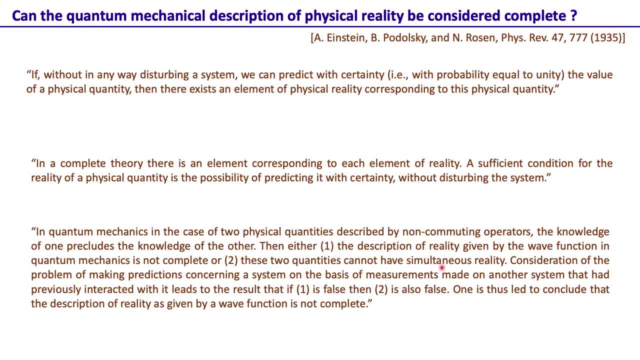 is not complete, or two. these two quantities cannot have simultaneous reality. Consideration of the problem of making predictions concerning a system on the basis of measurements made on another system that had previously interacted with it leads to the result that if one is false, then two is also false. 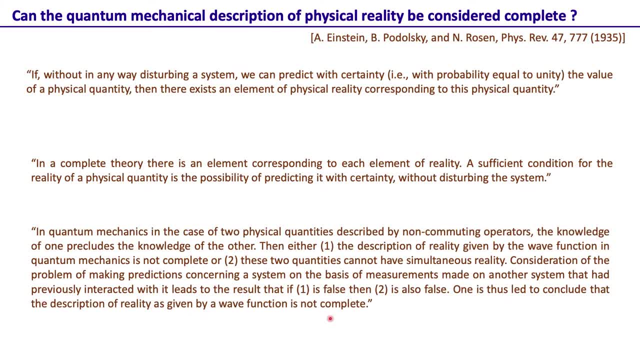 One is a slit to conclude that the description of reality as given by a wave function is not complete. Well, I will not go through this here. I just wanted to kind of point out these statements from the paper. but we will go through the paper now and through the maths to see what. 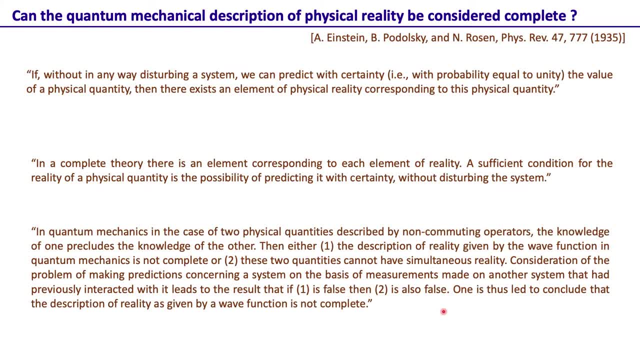 they are actually referring here, what they actually mean here. But one point is clear, which is what I wanted to kind of bring out here: that they were sort of feeling, and they were actually concluding, that the quantum theory as given in terms of wave function is not a complete theory, and they thought that something more. 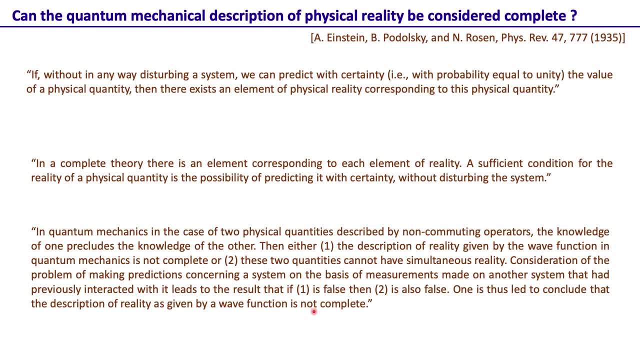 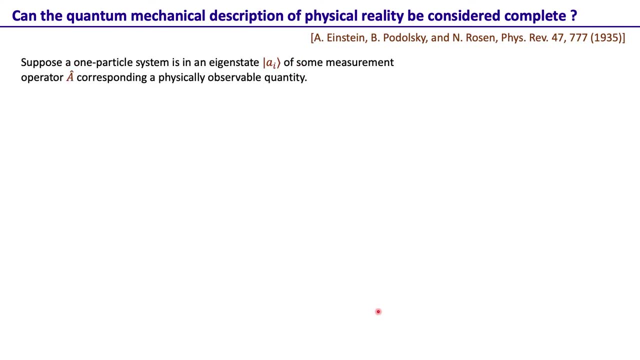 needs to be done with the theory. maybe some additional variables needs to be supplied to make it a complete theory. So now we will go through the math and arguments again, what they have done in this paper, to explain what they are pointing out here. So let's suppose we have a one particle system in an eigenstate AI of some. 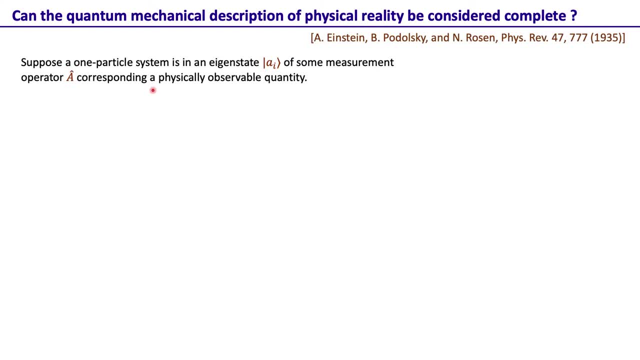 measurement operator, A corresponding to some physically observable quantity, Then we know that if A the operator acts on AI, which is the eigen ket, then we just get the eigen ket with eigen value AI, So the system remains unchanged, and further action of the A the operator on this state. 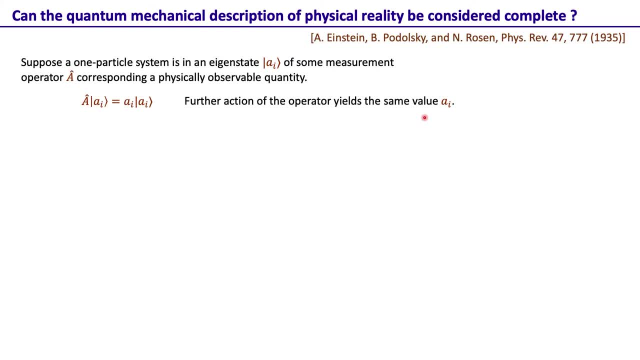 yields the same value- AI, because this is eigen ket, so the state doesn't change. So then we can say that there is an element of physical reality corresponding to some physical reality, corresponding to A. Now, this definition is coming from the arguments given, or the definition given by Einstein, Podolsky, Rosen, in the very beginning of the 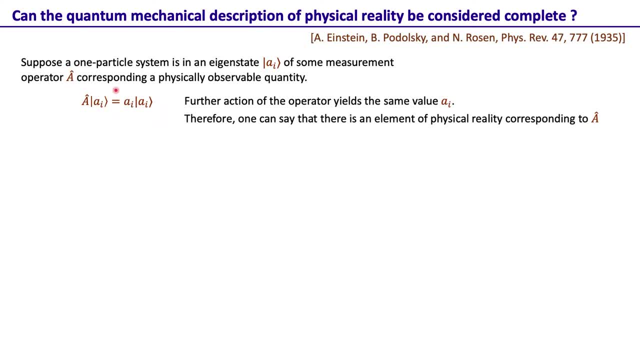 paper. So this situation? in quantum mechanics they identify that, yes, in this case we can say that there is an element of physical reality corresponding to A, because A acting A operator, A acting on this state, yields a value, AI, and if we just repeat the measurement, we get. 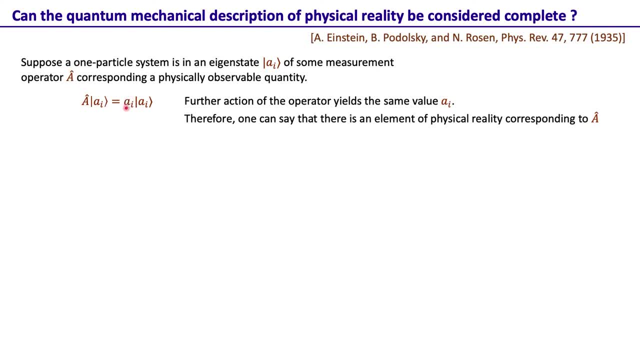 the same value. Okay, And then one could have predicted this with certainty even without this. A actually acted on this one. Okay, Now let's take a concrete example. So let's consider one particle system in one of the momentum eigen ket, For example. we can call it psi, p naught, and as a physical example we can see a photon. 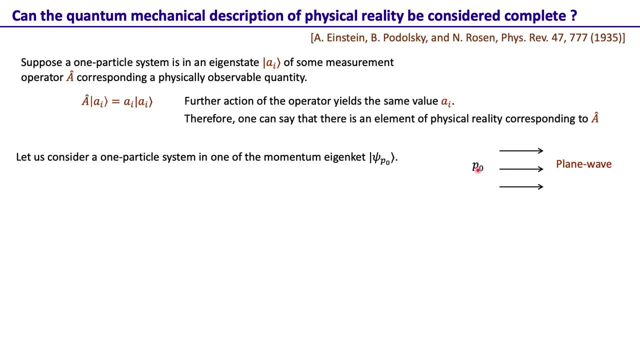 in a plane wave, a particle in a plane wave and with momentum, p naught and plane wave. that can be. that is a system with momentum. Okay, That is a system with in the momentum eigen ket. Now such a momentum eigen ket in the position basis we can find by taking the projection. 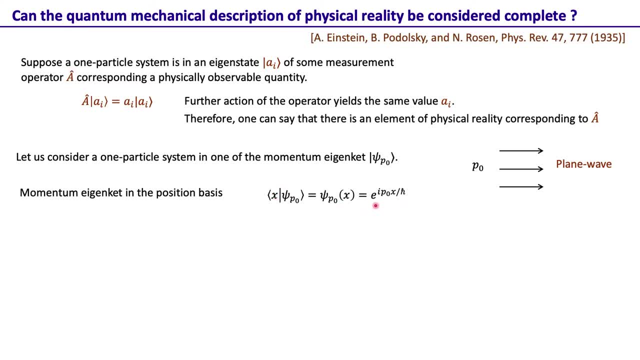 on the position basis, and we know, then this is given by this plane wave function, e to the i p naught, x by h bar, where p naught is a number, and that is the momentum of the one particle system. The momentum operator, in the position basis, we know it is given by this, is basic quantum. 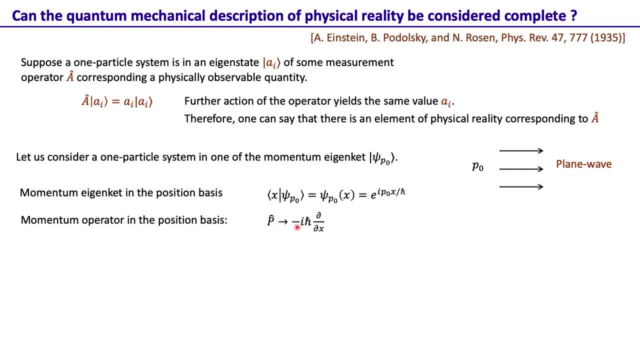 mechanics we are just doing here. Momentum operator in the position basis is minus i h bar del del x, and we know that the action of the momentum operator on the momentum eigen ket p acting on psi p naught, is that the state remains the same and we get the p naught out as the eigen value. 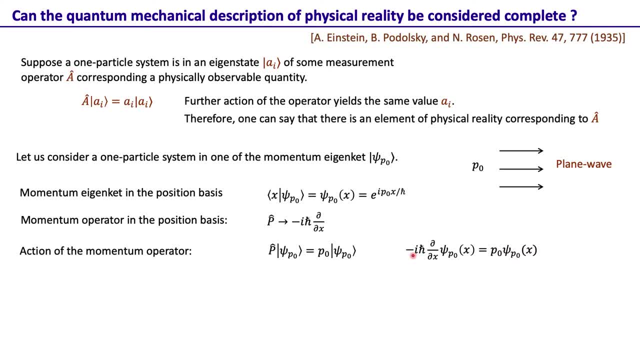 Of course this is in the state form. If you write in the wave function form, it is minus. i h bar del del x acting on psi p naught x, where psi p naught x is this: and so we get p naught out: i h bar del x. 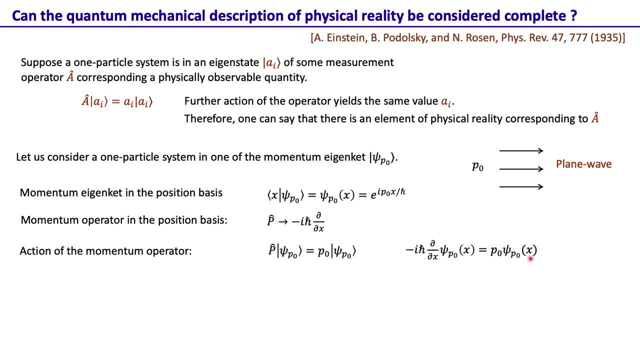 I by h bar p naught out and then so it's p naught psi, p naught x. So this is just getting the momentum value out. So what we see that for a system in one of the momentum eigen kets there is an element. 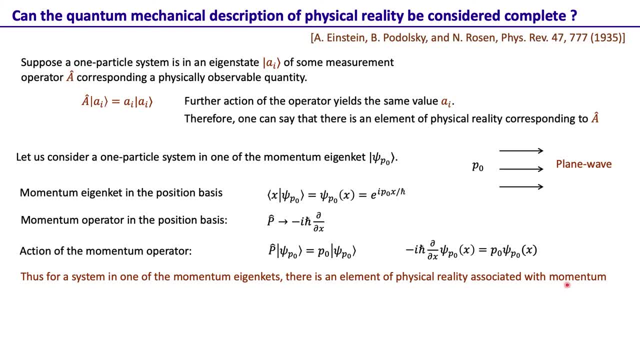 of physical reality associated with momentum. Why? because, without even disturbing the system, we could have predicted that we will get the momentum of the momentum value of p naught and that making a measurement doesn't doesn't change this value. and there is no uncertainty about about this, as to what value we would. 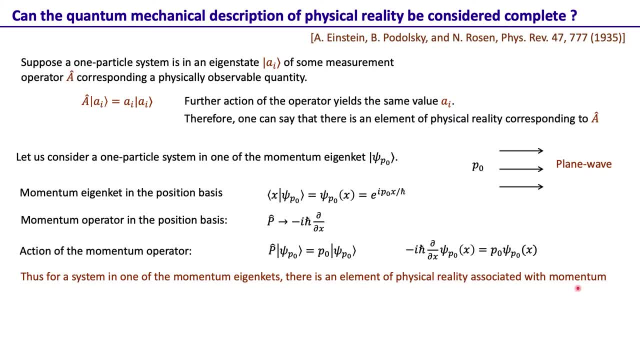 actually get. and that's why there is an element of physical reality associated with momentum for this particular system, which is one particular system in in the momentum eigen ket. that is a plane wave Now for such a system, what about the position now we know that for momentum eigen ket, if 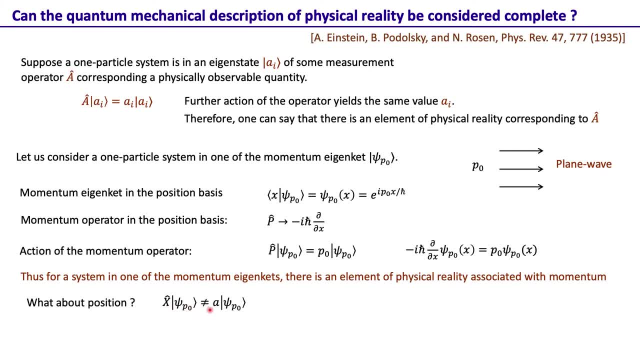 we act on it with the position operator. this is not of the form of an eigen value equation. that means we won't get psi, p naught And and times, times number. but we know that in this case what we can ask is basically the position probability. we can ask what is the probability that the particle is found? 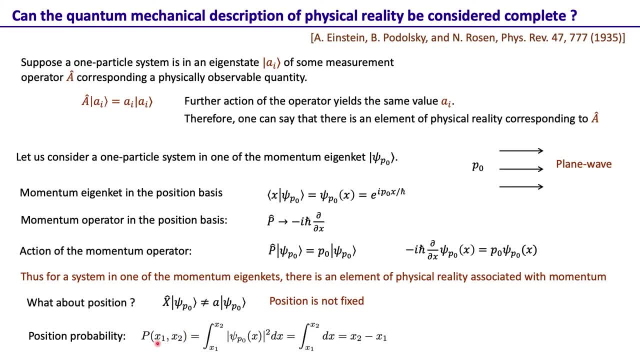 between position x 1 and x 2, and this we know that this can be obtained by using this position. probability density integrated over x from x 1 to x 2 and psi p naught x is has, has, has this form. So take the mod square is just 1, so that's just 1. so x 1 x 2 dx, that's x 2 minus x 1.. 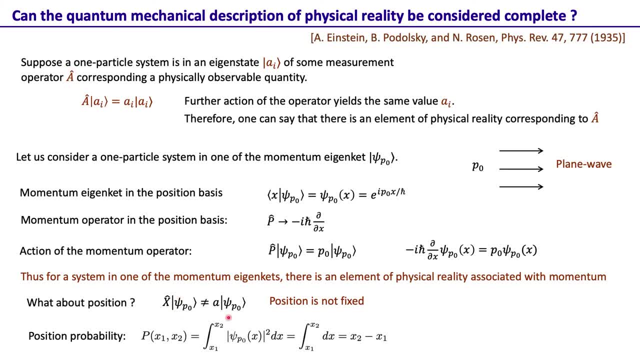 So the probability, so I mean an action of a position operator, this this tells us here that position is not fixed. all we can find is the position probability and the position probability between x 1 and x 2, that is, the, the probability that the particle is found. 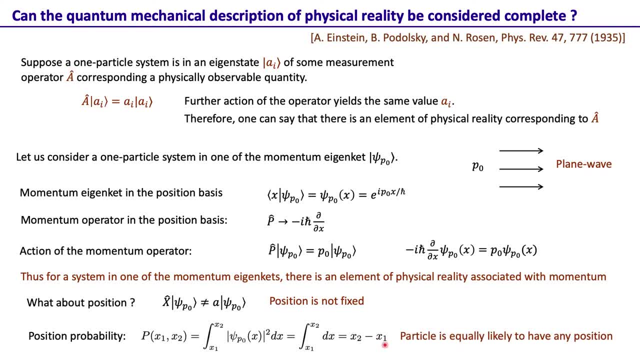 between position x 1 and x 2 is is just x 2 minus x 1. this essentially says the particle is equally likely to be found anywhere. So this one particle system in one of the momentum, eigen ket, has fixed momentum, but its position is completely uncertain. that means it can be. it is equally likely to be. 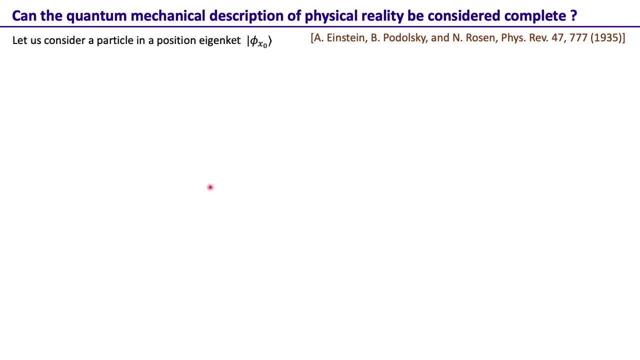 found at any position. ok, Now let's take another example, and this time we take a. we consider particle in a position, eigen ket, and as an example, we can see a wave diffracting from a point and that this is the x direction And that's the point x. 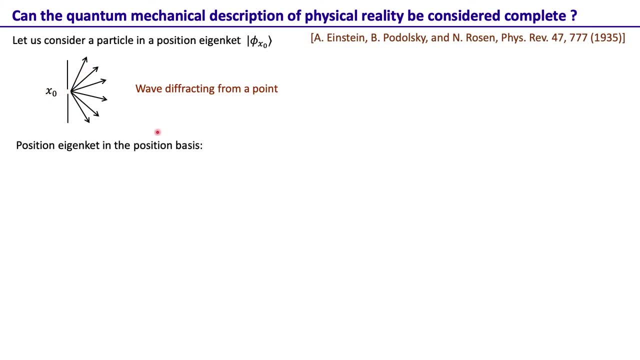 Not from where this, this wave is coming. So now I mean this: this is: this is one very- this is physically realizable- example of a kind of position eigen ket, Now position eigen ket in the position basis, to a very good approximation. we can, we can. 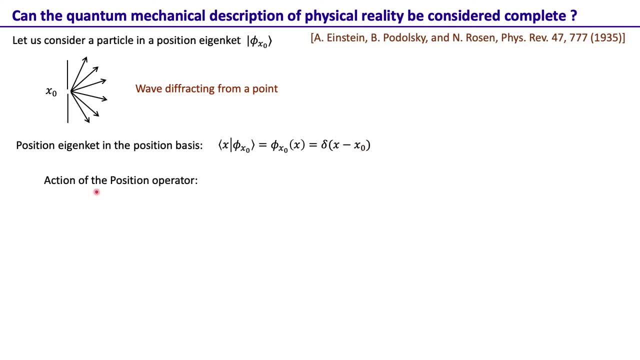 write that as a delta function, delta x minus x naught and action of the position operator on on this wave function is that, since this is a position eigen ket, we of course get the same state And this x naught. This is a value, eigen value that we get out. 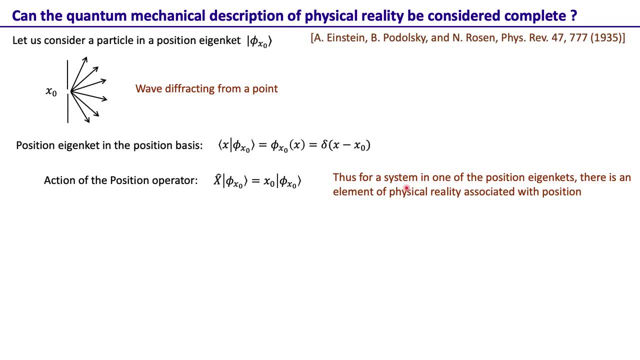 So, in this case, the system being in one of the position, eigen ket- there is an element of physical reality associated with position. and when we say element of physical reality, this is as: according to Einstein, Podolsky, according to the definitions by Einstein, Podolsky and Rosen, 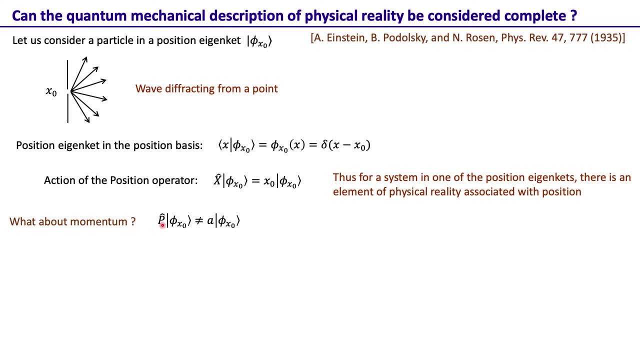 So now, in this case, what about momentum? of course, if we, if we act the momentum operator on this position, eigen ket- then of course we do not get it like this. So this equation is not. that doesn't have any meaning. So all we can say is that the momentum is not fixed. 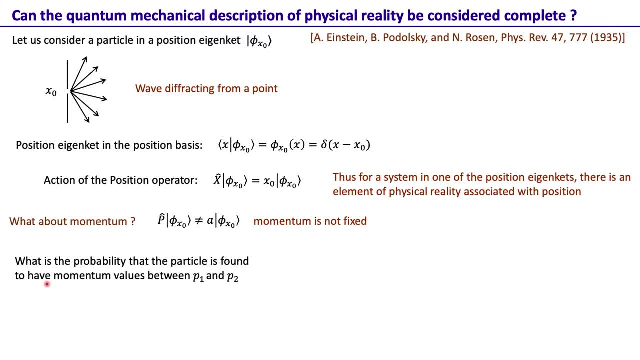 but then the question is: what is the probability that the particle is found to have momentum values between P1 and P2?? And again, we can do the same math. So the probability that the particle has momentum between P1 and P2 is just the momentum wave function. 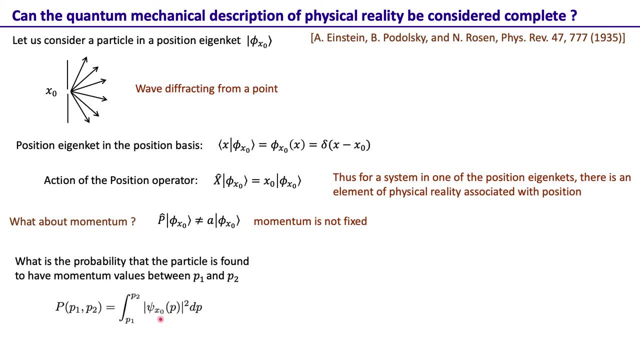 that is whole, squared, that is the momentum probability density and integrated from P1 to P2.. So what is psi x naught p? Well, psi x naught p we can calculate because we know the wave function in the position basis. So, knowing the wave function in the position basis, 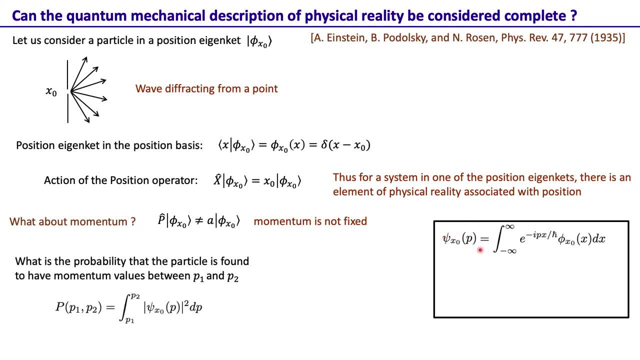 we take the Fourier transform and then we can get the wave function in the momentum basis, Since the wave function in the position basis is a delta function that we can just put in here and that gives us that the wave function in the momentum basis corresponding to this wave function. 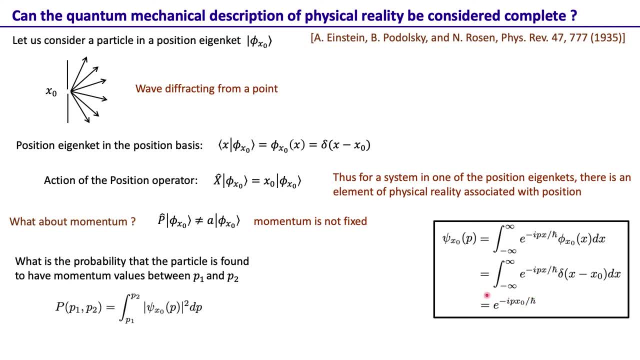 is e to the minus, i p x, naught by h bar. So if we now, if we just take the absolute square of it, this is essentially one, And so that's why this quantity is P1, P2, dp, that is, P2 minus P1.. 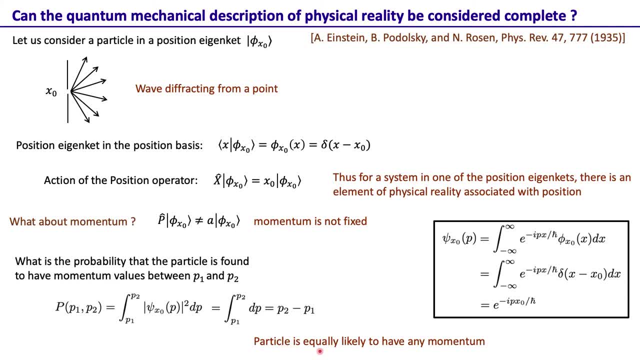 So again we have here: this particle is equally likely to have any momentum. So a particle that is in a position I can get with this wave function. its position is fixed and that is at x is zero, but the system or the particle 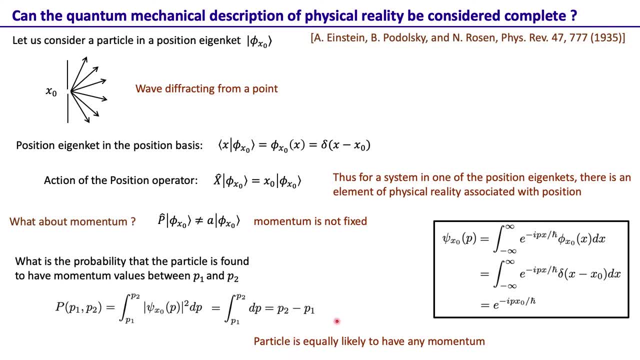 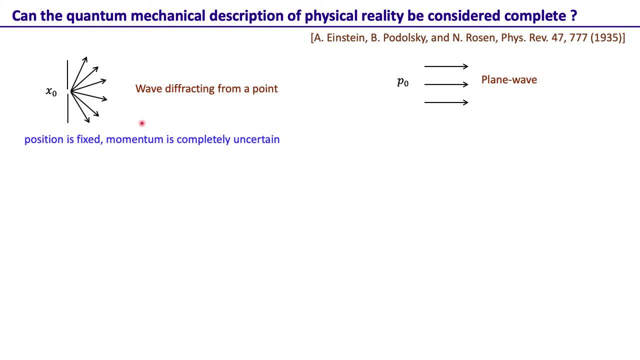 is equally likely to have any momentum value. Okay, so what we have done so far is that for a wave, for this example, where we have a system in a position I can get, position is fixed and momentum is completely uncertain- This we can write as delta. 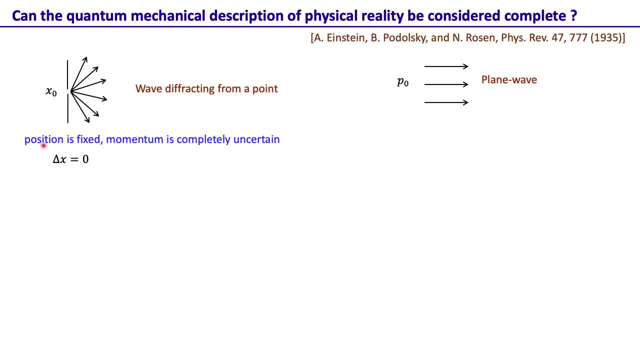 Delta x, that is uncertainty in x, that is equal to zero, because position is of course fixed, but the uncertainty in p, that is, momentum, is infinity. Similarly, for our plane wave example, the momentum is fixed and position is completely uncertain. 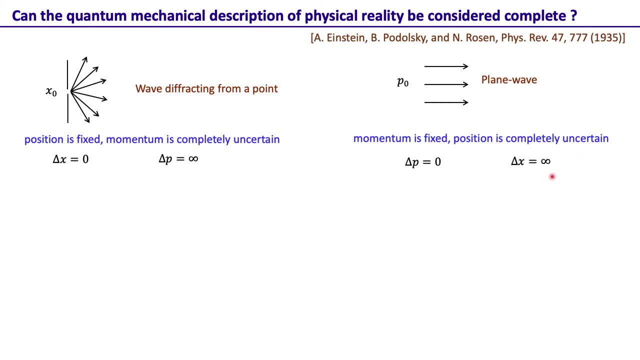 That means the uncertainty in p is zero and the uncertainty in x is infinite. But this was just one set of example. but in general we know that in quantum mechanics we have delta x times delta p is greater than h bar by two. 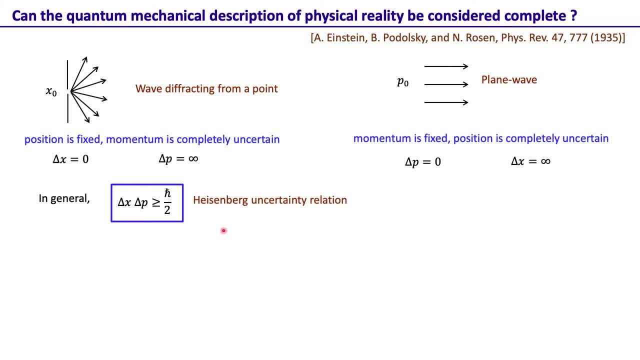 And this is called the Heisenberg uncertainty relation. This basically says that two non-commuting operators, such as position and momentum, and if they don't commute, for example x and p, not equal to zero. So for such a case, 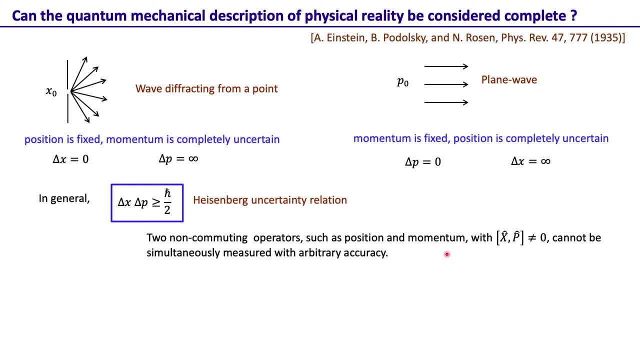 they cannot be simultaneously measured with arbitrary accuracy. The position and momentum: these cannot be measured with arbitrary accuracy. If we know one very accurately, then our knowledge of the other one will not be as accurate. Of course, these two are extreme examples when we're, in this case, we know x very, very accurately. 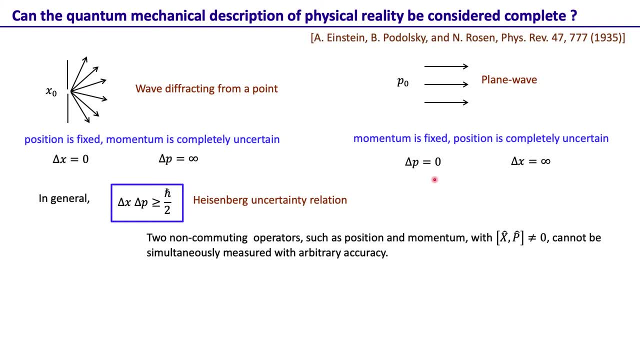 And so we just don't know anything about p. In this example, we know p very accurately and hence we know nothing about the position, I mean, as it can be anywhere. Here the measurement accuracies are dictated by the uncertainty relation. 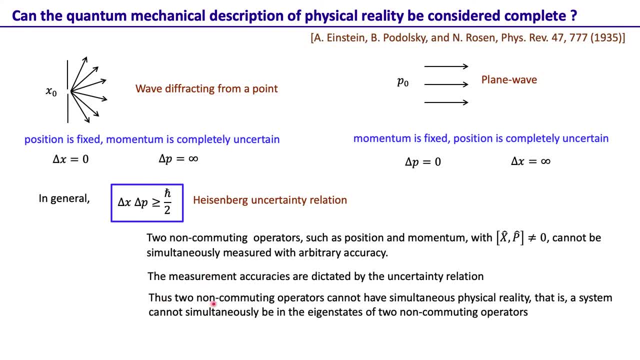 And so I mean, in other words, we can also say that the two non-commuting operators cannot have simultaneous physical reality, That is, a system cannot simultaneously be in the eigenstates of two non-commuting operators, Because if it is in the eigenstate of position, 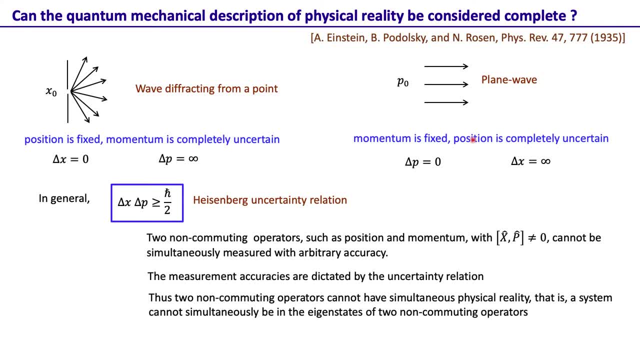 then of course delta x is zero, And if it's an eigenstate of momentum, then of course delta p is zero. So system cannot simultaneously be in the eigenstate of two non-commuting operators. So this is all standard quantity. 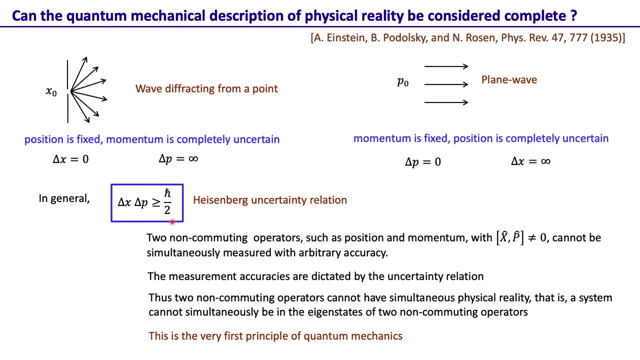 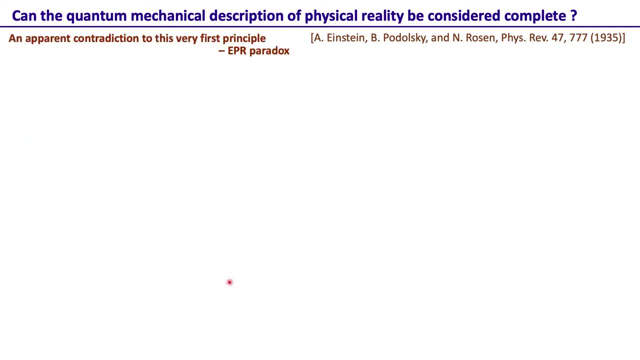 And this is this uncertainty principle in this form and with this interpretation- is: this is the very first principle of quantum mechanics. Now, Einstein, Podolsky and Rosen, they basically took this very first principle and then, using this first principle, they actually saw an apparent contradiction. 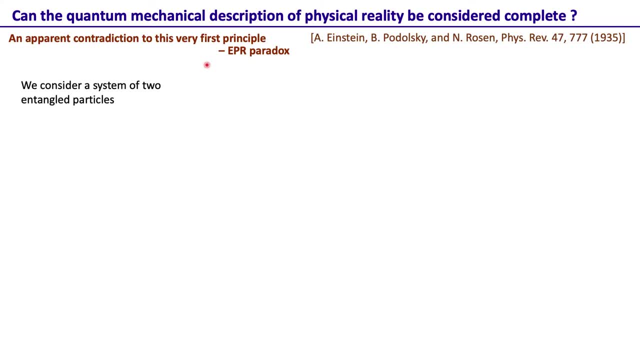 within the quantum theory, And that's what we will calculate, describe now. So for this, let's consider a system of two particles, two entangled particles. These particles had a common path. That means they interacted in the past And then, but after that they separated. 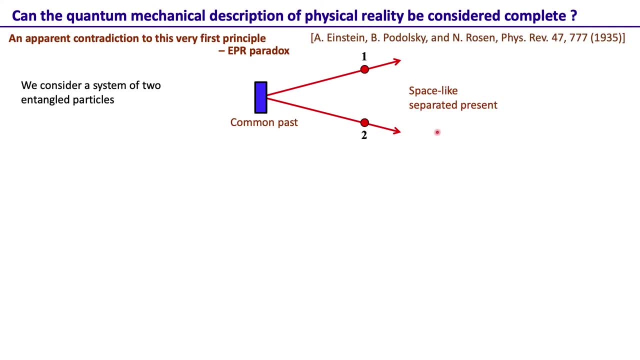 And now they are space-like. the present is space-like, separated, So now there's no interaction after they have separated. So I mean they can be any wave function, but let's assume that I mean this is the wave function considered by EPR in this paper. 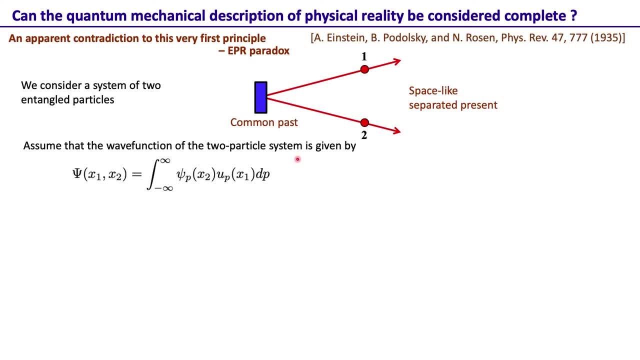 So they assume they just take a wave function for this two particle system in this form in the position basis. So psi x1, x2 is a psi p, x2, up, x1, dp. This is for the first particle and this 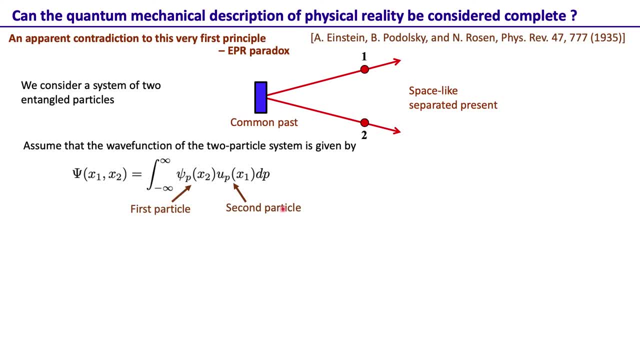 is for the second particle. So that's a wave function corresponding to first particle, That's a wave function corresponding to the second particle. So we see that this is a continuous superposition of two particle states. So this two-particular state is a continuous superposition. 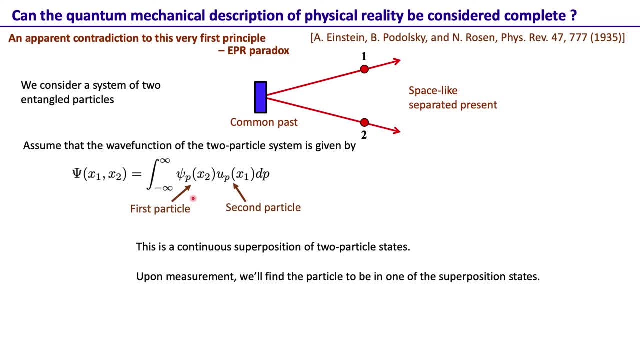 of such two-particle states. And upon measuring the two-particle state, if we actually go and measure it, we'll find- and this is what we did in the last lecture on quantum measurement. So this is a superposition of many such states. 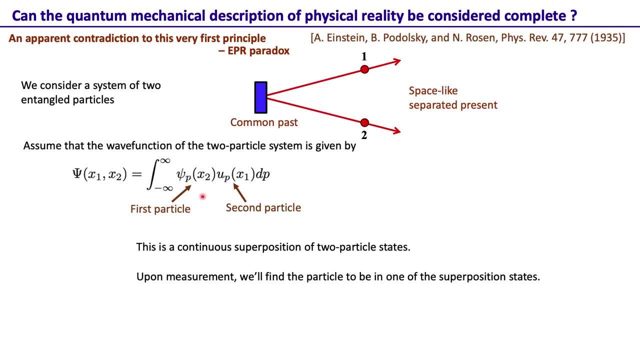 defined by this index p here, And so if you make a measurement, we'll find just one of these terms: psi, p, x2, up x1.. So upon measurement we won't find this entire integral, We'll just find the state of our system. 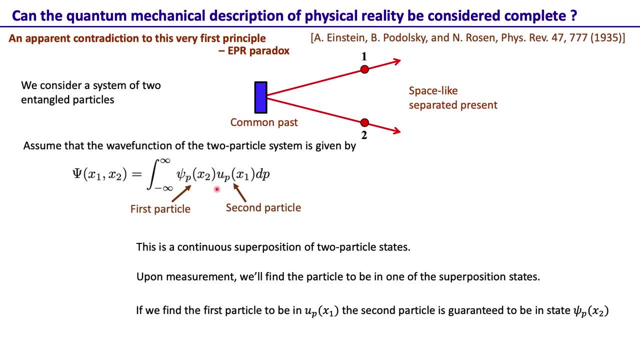 to be in one of the superposition states, And so the thing is now: if you find the first particle to be in up x, then the second particle is guaranteed to be in psi p x2.. So this state is fixed by this index p. 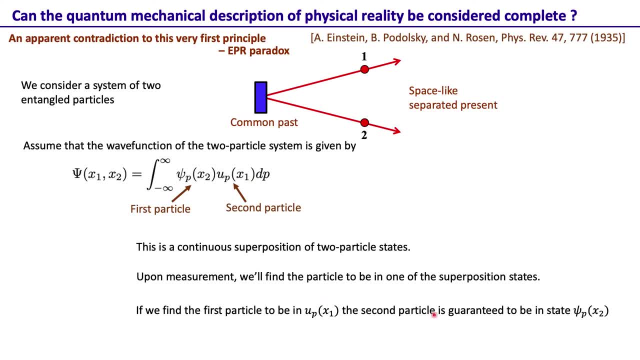 Of course, if you find the first particle to be with up prime x1,, then the second one is guaranteed to be in psi, p prime x2, as it is an integral over p. OK, So this is a generic, OK, Generic wave function. let's make it more precise. 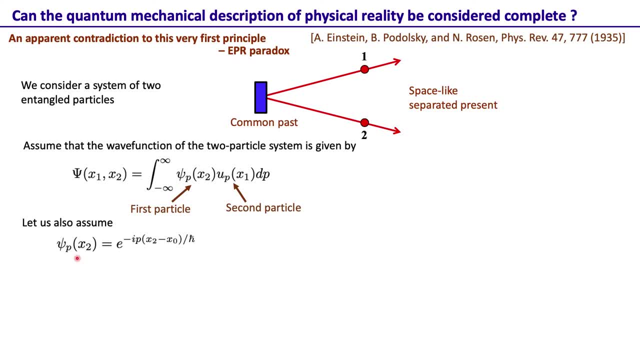 So for that, they actually consider this wave function. So for psi, p, x2, they consider it to be in this form, And up x1, they consider it to be in this form. Now, what is this wave function? This we have just done a few slides ago. 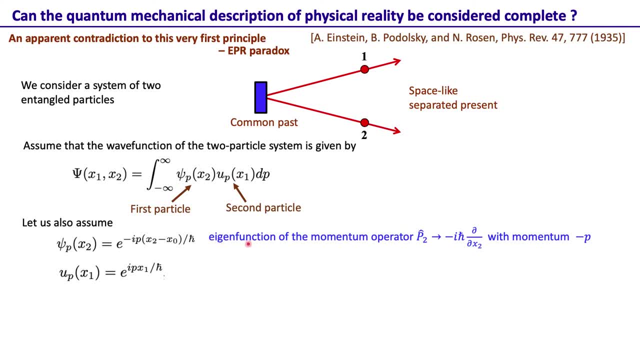 This is a wave function. This is essentially an eigenfunction of this e to the minus ip, x2 minus x1.. Of course, we can take any form for these wave function, but EPR took this form because this is the simplest and conveys the main idea. 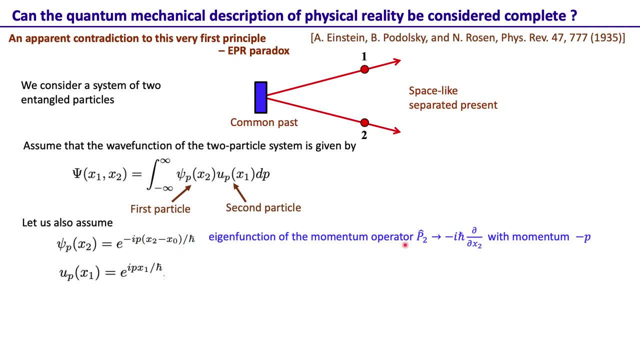 So for this one, this, we see that this is an eigenfunction of the momentum operator of the second particle, that is p2.. And this, we can see that this minus ih bar del del x2, if we just act on it, we get minus p out and this stays. 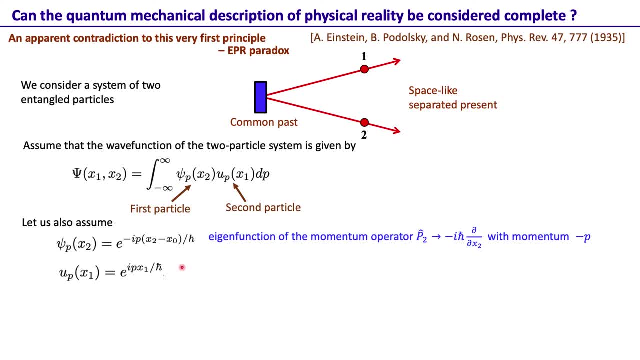 So this is an eigenfunction of the momentum operator of the second particle. What about this? This is actually an eigenfunction of the momentum operator of the first particle And the momentum operator is given by minus ih bar del del x1.. So we can see if we operate minus ih bar del del x1 on this one. 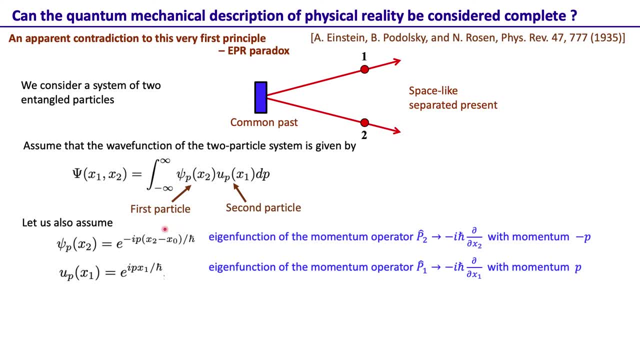 we get p out and the state remains. So this is an eigenfunction of the momentum operator of the second particle and it gives the momentum minus p. This is an eigenfunction of the momentum operator of the first particle with eigenvalue p. 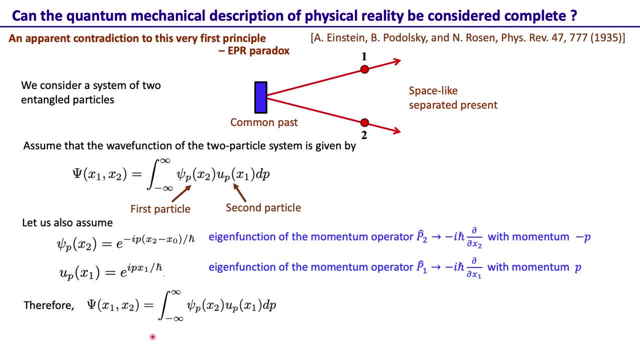 This one is minus p, This one is p. So we can do this. We can write this state for this particular example. We can write the state like this, And the interpretation that we have is that, of course, this is an integral over a p. 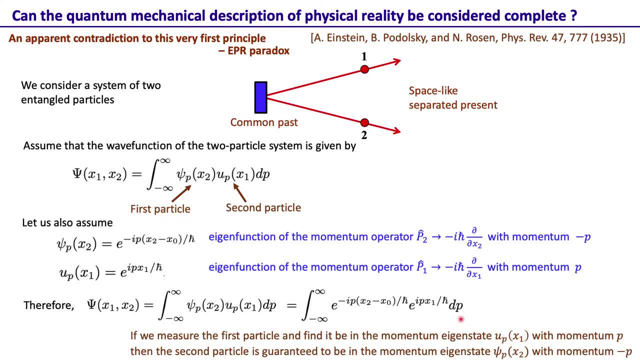 That is a summation, That is a superposition, is given in the form of the integral And, of course, if you make a measurement, then, as we discuss here, it has to be. this two-particle system will collapse into one of these states that are part of this superposition. 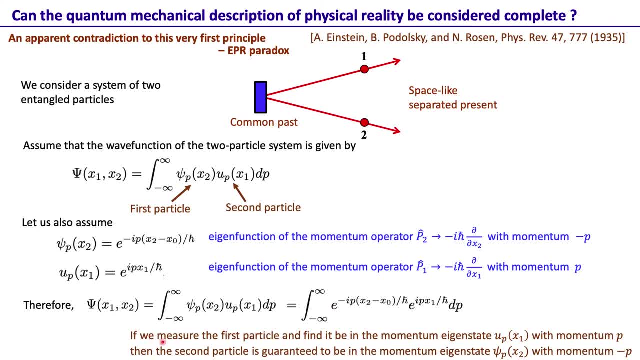 So if you make a measurement, you're going to get p. So if you make a measurement, if you measure the first particle and find it to be in the momentum eigenstate u, p x, 1 with momentum p, then the second particle is guaranteed to be in the momentum eigenstate psi, p x. 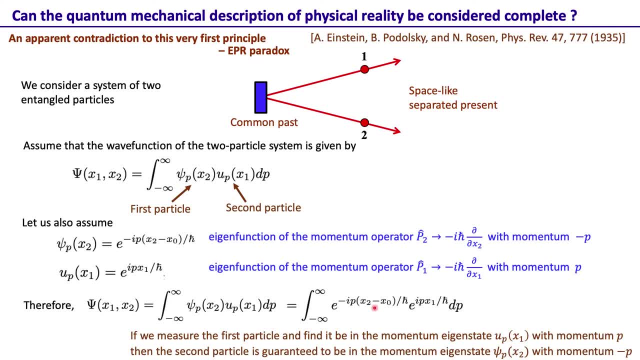 with momentum minus p. So what we find is that, of course, each particle can have any momentum value, But if you find the first particle to be with momentum p, then the second one is guaranteed to have momentum minus p. OK, so that's the situation. 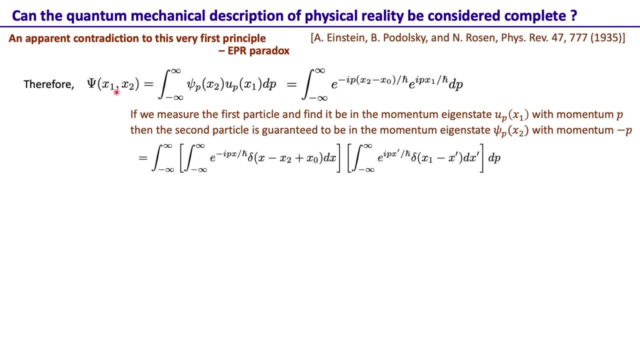 Now what we do is we can: let's write this state Right now. this one is in the momentum basis and with this particular example, Now let's write this state, which is in the momentum basis, in the position basis For that, this e to the minus i, p, x 2, minus x 0 by h bar. 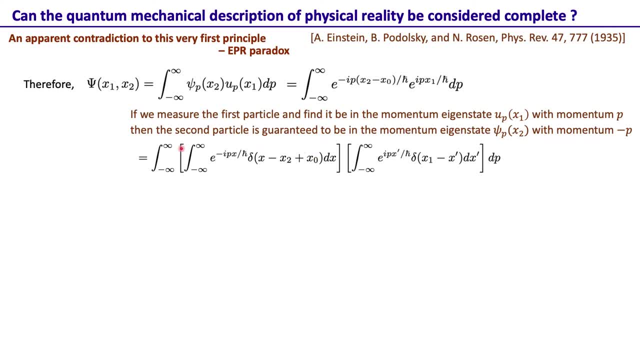 that is the wave function for the second particle. Let's write it like this: So we're just writing e to the minus i, p x 2, minus x 0. OK, OK, So we can write this as an integral over: x. 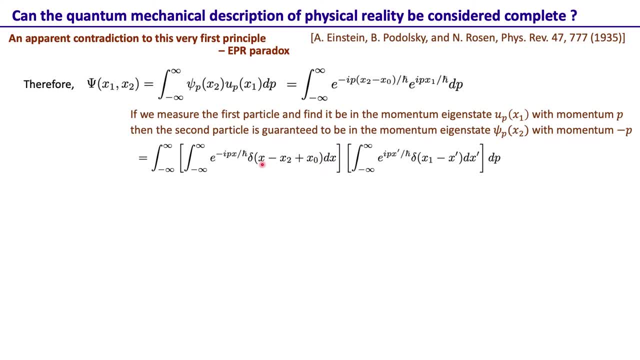 And that's the delta function. comes here We can check: if we just integrate over this, This delta function goes away And we can replace this x by x 2 minus x 0.. Similarly, this e to the i p, x 1 by h bar. 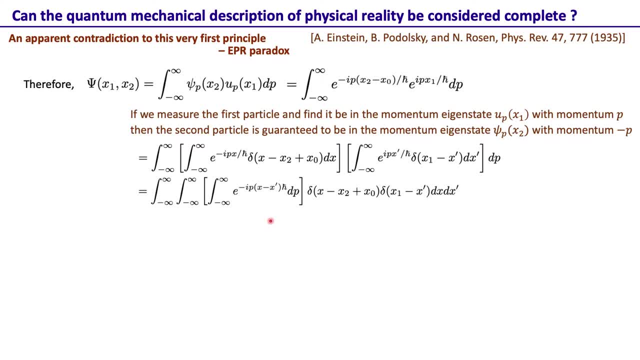 that can be written as an integral over this dx prime in this manner. OK, so now that we have written this integral like this, we combine the terms containing p So: one from here, one from there, One from here, one from here, one from there, one from here. 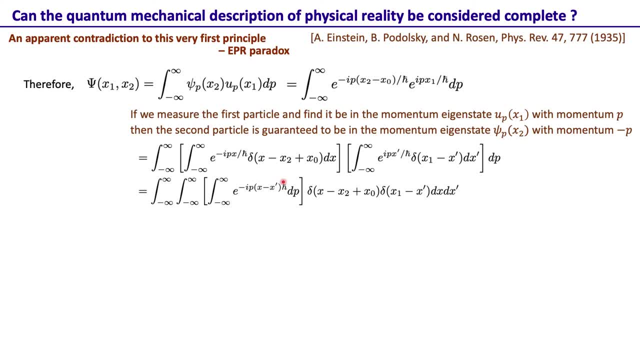 And then we have this integral over x bar x minus x prime. Oh, this should be divided by h bar dp. And then we have these two delta functions: Now e to the minus i p, x minus x prime. that actually gives us an integrated minus infinity. 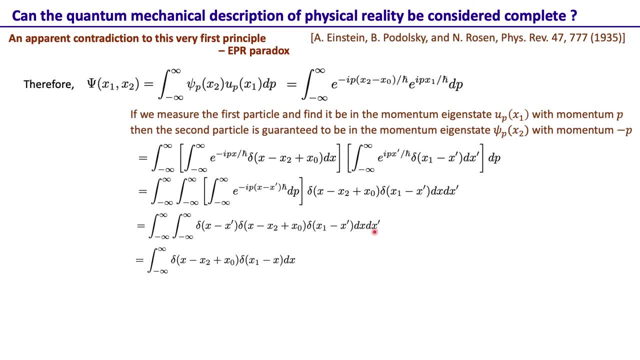 This actually gives us a delta function: x minus x prime. So we have three delta function and two integrals over dx and dx prime. We integrate over dx prime. This is the product of two Dirac delta function, So the same state which in the momentum basis. 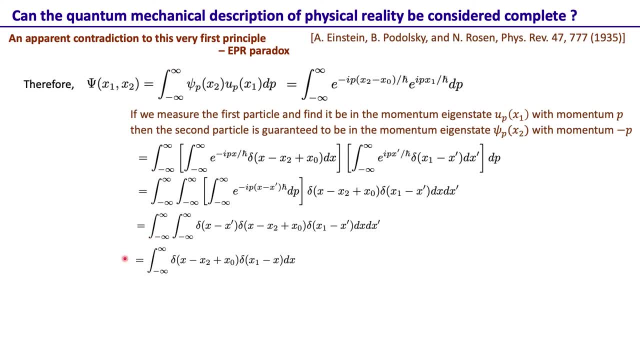 has this kind of representation. the same state in the position has this kind of representation. Now, when this has this kind of representation, this again corresponds to: this is a wave function corresponding to particle number 2. And this is a wave function corresponding. 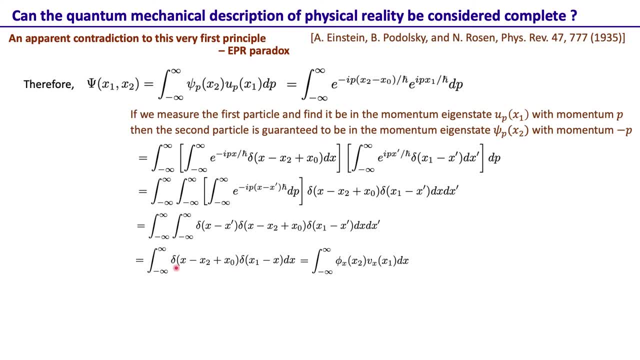 to particle number 1.. We can also call it psi. This one, we can call it as a phi x x 2.. And this one, we can call it as v x x 1.. Now, what is this? delta x minus x 2. 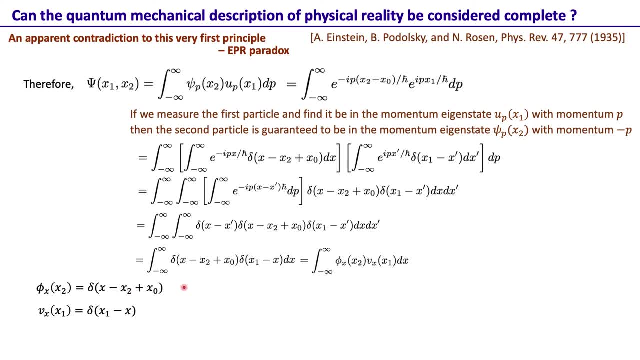 plus x naught. Now this delta x minus x, 2 plus x naught is essentially the eigenfunction of the position operator of the second particle with the eigenvalue x plus x naught. This again we had seen when we were discussing the position. 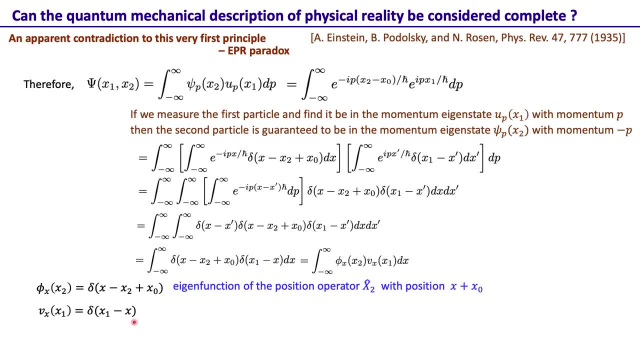 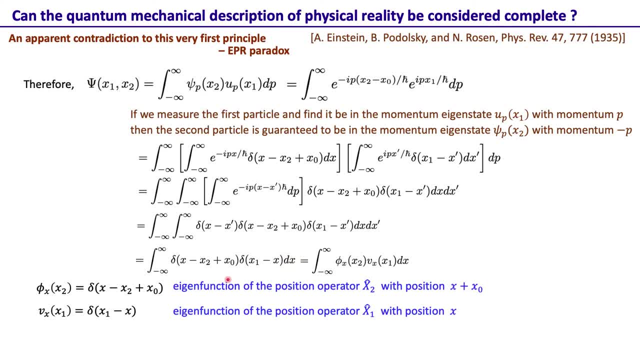 Again, this is an integral over dx. That means this state we are representing as a superposition over this x. But of course, when we make a measurement, we will not, we will. the system will collapse into one of the terms in the superposition. 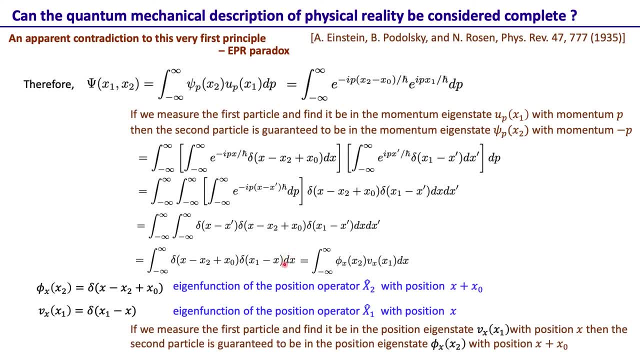 And as a result, we will see that of course we can. we can get any x value, But once we make a measurement and if we find the first particle to be in the position eigenstate, v, x, x, 1 with position x, x and the second one is guaranteed to be in the position eigen state with eigen value. 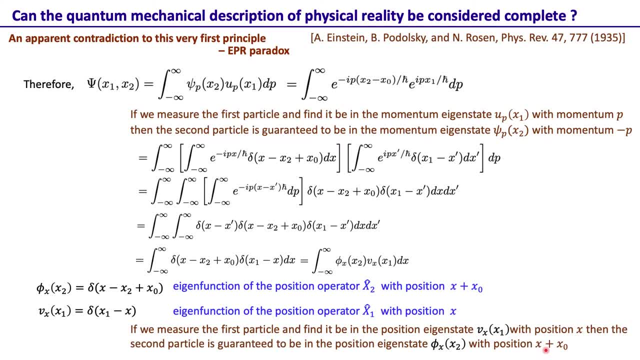 x plus x naught. So again, upon measurement, any x value is possible from negative infinity to infinity. but if the first one has a position, if the first one is measured to be at position x, then the second one is guaranteed to be at position x plus x naught. So what we have? 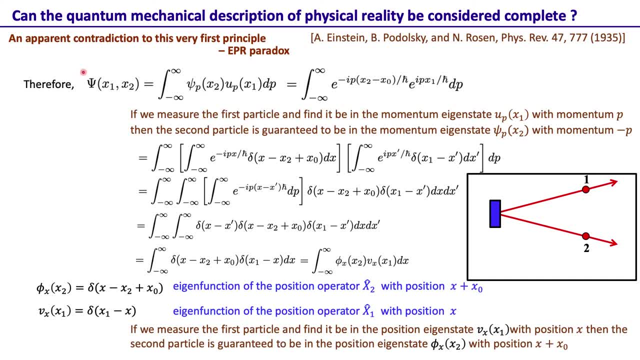 here is that we have in the for the same wave function, So for the same system. we find that if we make a measurement of the momentum of the first particle and if we find that momentum to be p, then the second particle is found to be with momentum minus p. but 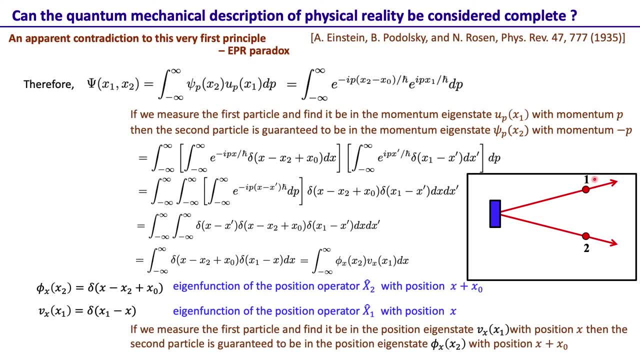 if we decide to look at the position of the second wave function, then the second wave of the first particle, and then we find that its position is x, then the position of the second particle is found to be x plus x- naught, Of course. this is this minus p. this is the 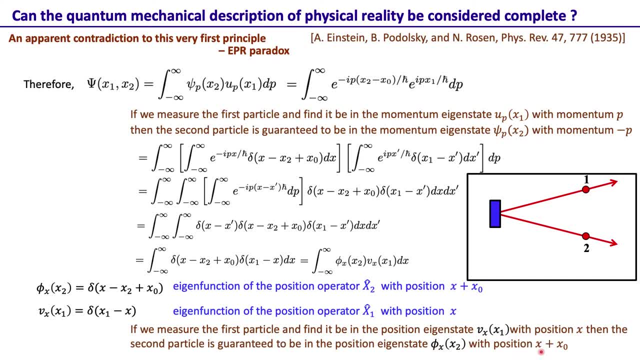 momentum eigen state, and this is state with x plus x naught eigen. this is the position eigen ket. So it seems that by our choice of measurement is deciding whether the state of the particle here is a position momentum eigen ket or a position eigen ket. 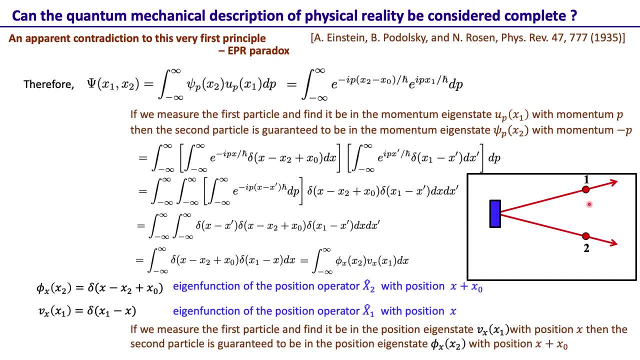 So in other sense we can also say that if once we make the measurement of the momentum here p, then the momentum of the second particle is fixed. but if we decide to make a position, measurement in the position of the second particle is fixed. So what we here have is: 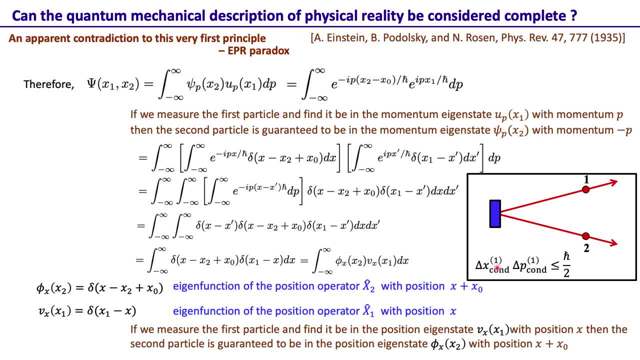 this conditional uncertainty on the particle, on the second particle based on the measurement already done on first Times, the conditional momentum uncertainty of the second particle based on the measurement already done on the first particle. this can, at least in this example it can- actually be 0. So that means this product can actually be less than equal to h bar by 2, which is: 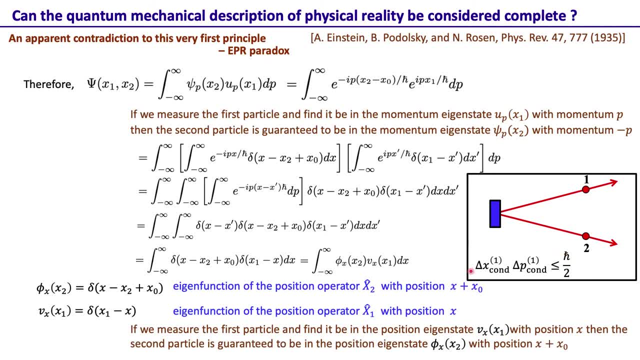 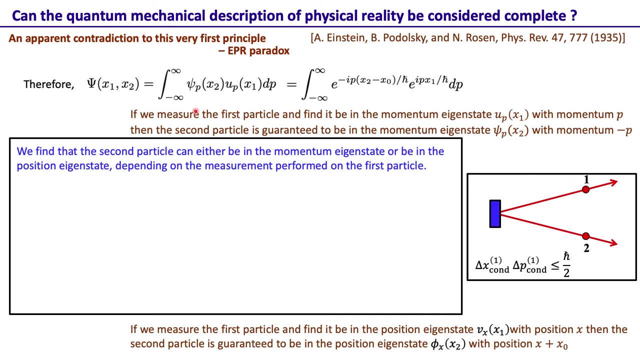 the Heisenberg uncertainty relation. So this was the feature. they pointed out that for such a wave function, which is definitely allowed within quantum mechanics, we have this interpretation. this is in contradiction to what we saw for the very first wave function, So EPR then interpreted this as well. these are the facts that actually come out when 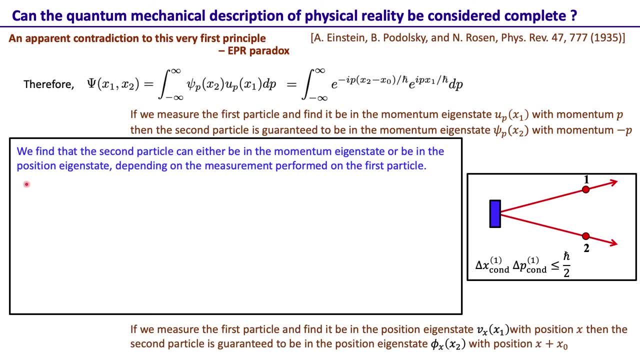 we construct these function and see what happens upon measurement. So they basically concluded that yes, we find that the second particle can either be in the momentum eigen state or be in the position eigen state, depending on the measurement performed on the first particle. So a measurement on the first particle decides. 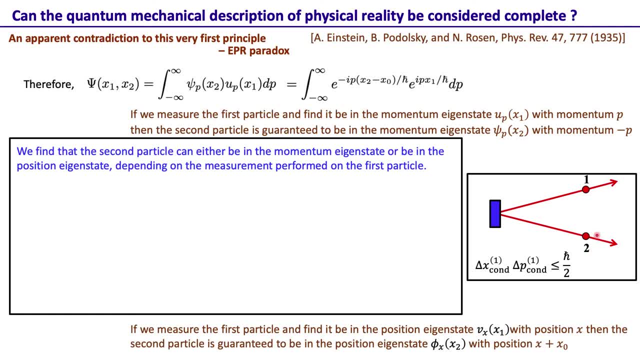 whether the second particle will be in the position eigen state or in the momentum eigen state. and here we need to note that the particles once they have separated, there is no interaction between them. there is no other measurement or disturbance that this particle has seen. it is just that a measurement on this particle is deciding whether this particle is in position. 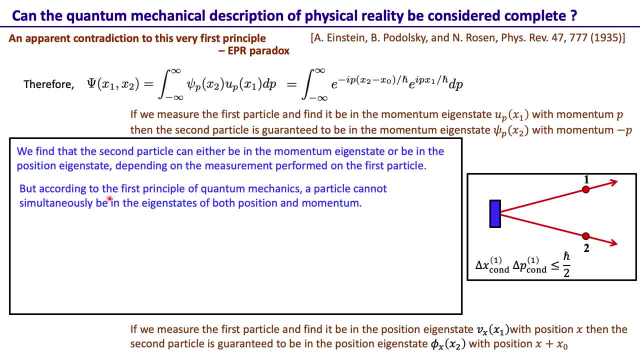 eigen state or in momentum eigen state. But according to the first principle of quantum mechanics a particle cannot simultaneously be in the eigen states of both position and momentum. So of course this particle cannot be in the simultaneous eigen state. So a, so it looks it, so it seems that a measurement here, the choice of the measurement, is kind. 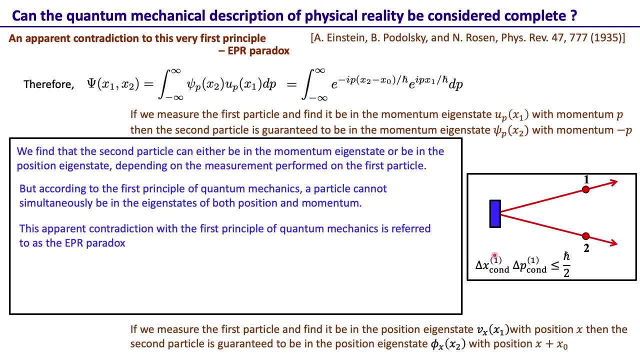 of collapsing this particle into either position or momentum eigen state, which is in contradiction, apparent contradiction, with the first principle of quantum mechanics. And this fact, this apparent contradiction this is, this is referred to as EPR paradox, so that. So that was the gist of that paper and their argument that I had in the very first slide. 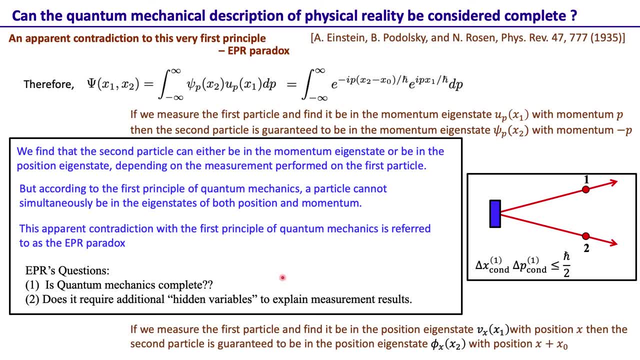 So, with these observations, basically then the question that if this is the feature that we see within quantum mechanics, that the first principle says that one cannot have a particle or a system cannot have been simultaneously, cannot simultaneously have the two eigen kets, but if we consider a two particle system, then we do have a situation where we find 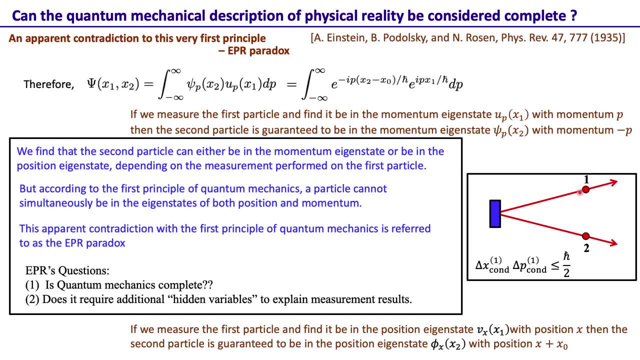 that a measurement performed on the first particle collapses the system into either one eigen ket or in the second eigen ket of two non-commuting operators, and the only way this can be explained is perhaps by saying that this particle probably exists or probably has the simultaneous eigen. 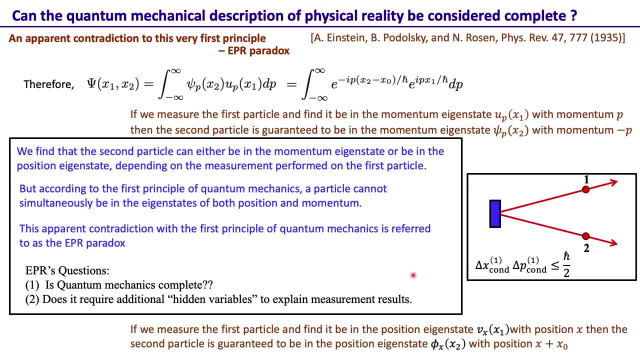 ket, Which is again in contradiction with the first principle. So with these observations, basically, the question: is quantum mechanics really complete? and if it is- or maybe it is complete, but it may be- it requires some additional hidden variables to properly explain the measurement results.